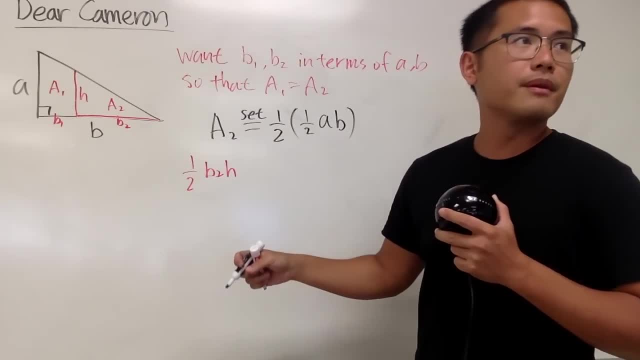 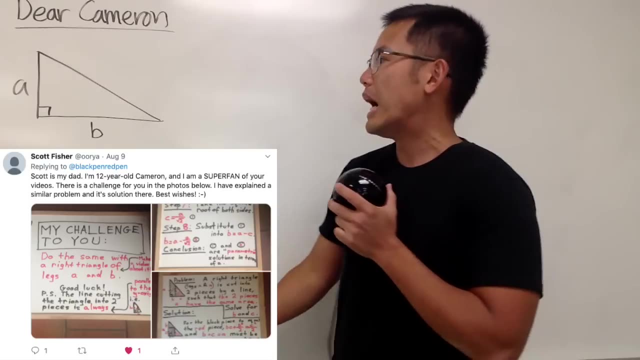 B2 times H, like this: Okay, Cameron, this right here is for you. We have a right triangle like this, And your question is that: how can we make a vertical cut somewhere? And let me just draw a vertical cut. Let me just put it down like this: 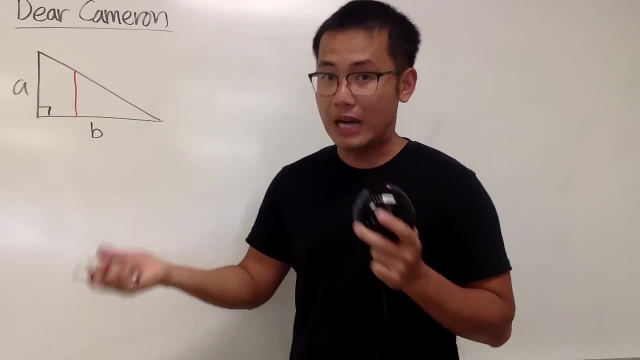 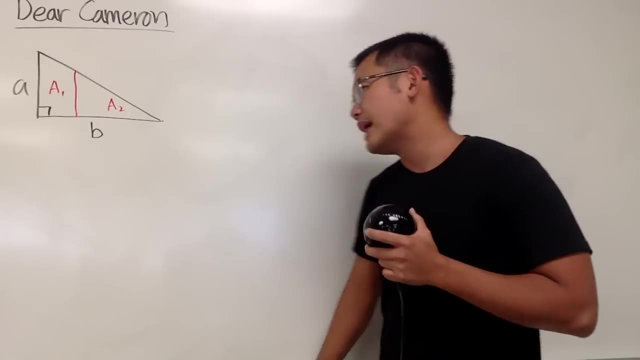 And we want this piece and that piece to have the same area. So perhaps I'll just call this piece right here to be A1, and this piece right here to be A2.. And how can we make this happen, right? Right, Since the question is asking us. 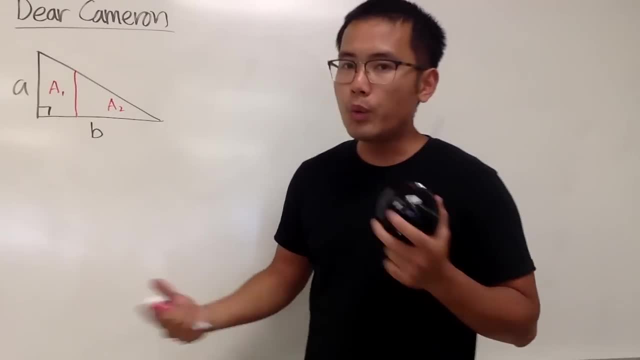 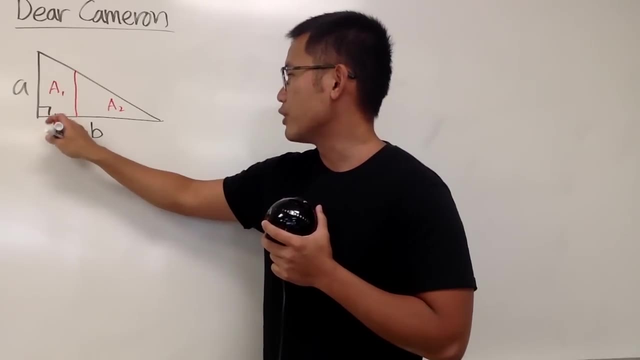 how can we make a vertical cut like this? Perhaps one way to answer it is, of course, we can just tell the distance from here to here and the distance from here to here. So perhaps let's just call this right here to be B1,. 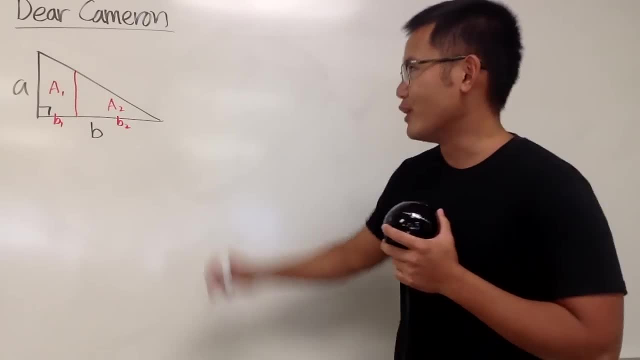 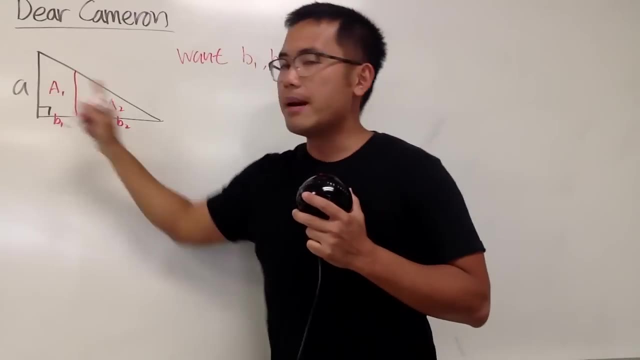 and this right here to be B2.. So here is the deal. This is what we want. We want B1 and B2, and because we were given A and B, so B1 and B2 have to be in terms of A and B. 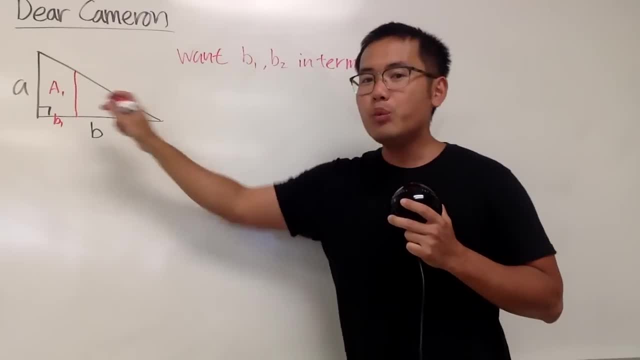 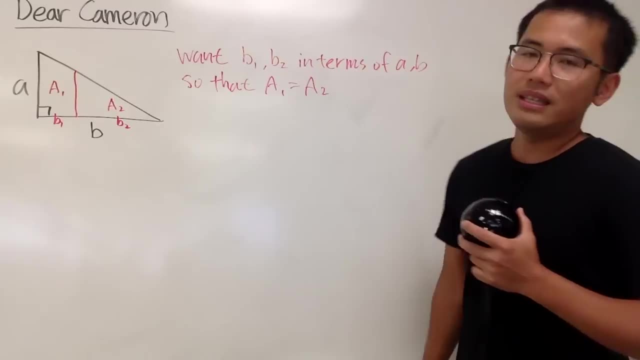 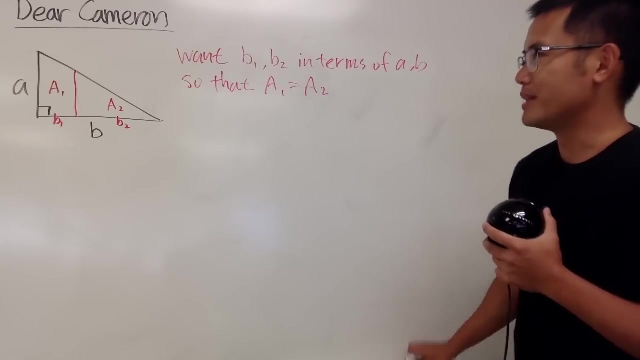 and, of course, our goal is to make sure that A1 is equal to A2.. So we want to put down: A1 is equal to A2.. This is our goal, right? Hmm, how can we make this happen? Well, well, let's think about it a little bit. 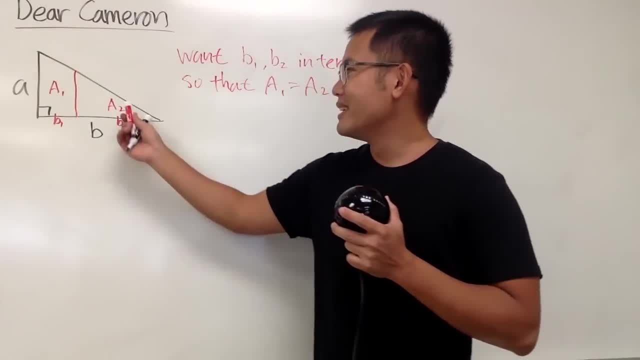 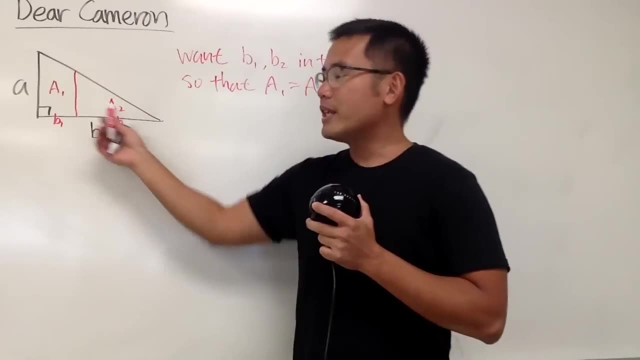 If this and that have the same area, of course, let's just look at this one right here, because A2 is just a small right triangle, so that's very nice right. This right here will just have to be half of the original triangle, isn't it? 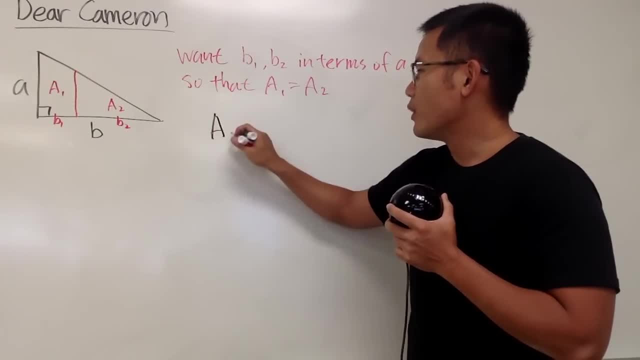 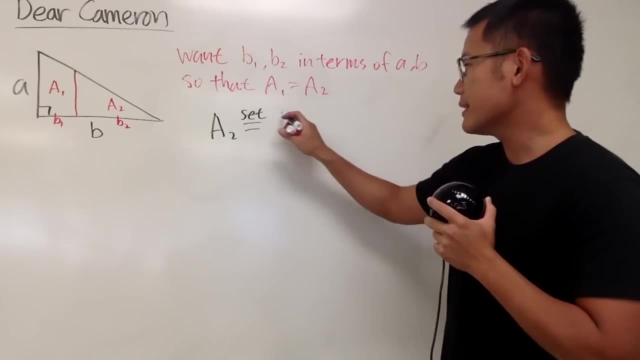 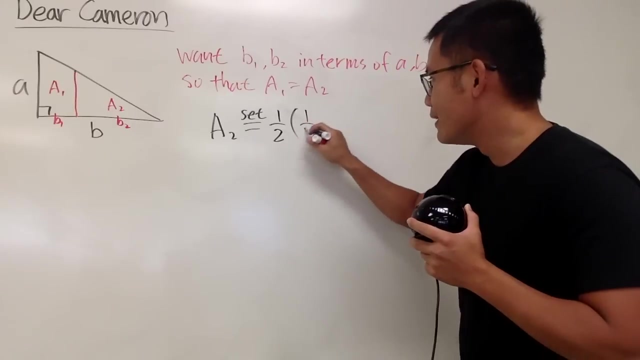 So here is the deal. This is the idea. We want to first set A2 to be just half of the original triangle. So now let's put that down. We want one half, and the area of the whole triangle is again half times. let's take this for the base. 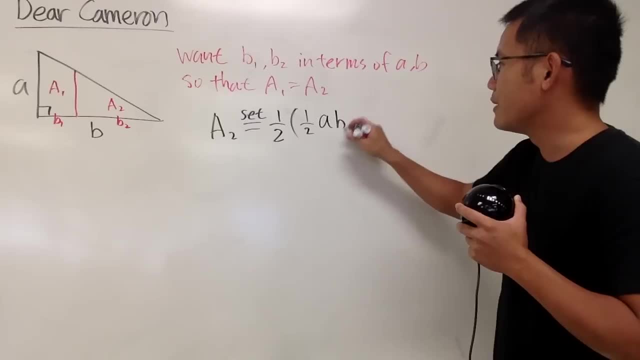 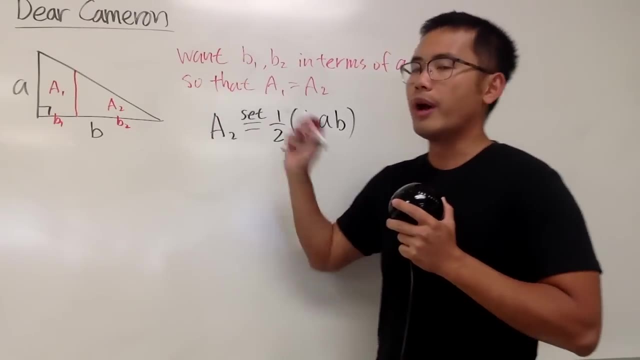 and take that for the height, so we have just AB right, So half of AB. like this. This is what we want to achieve. Perhaps let's look back here to see if we can come up with another formula for A2.. 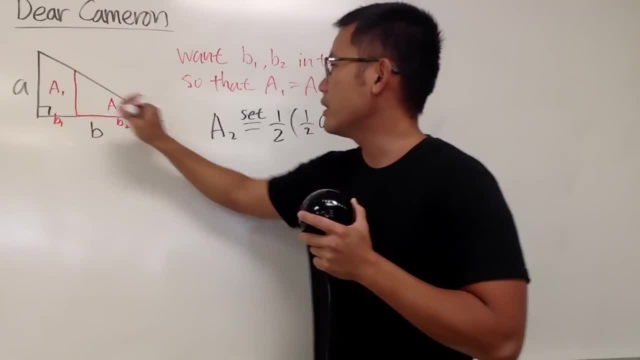 Well, as you can see, A2 is just this right here, this right here, and that right here. It's just a small triangle, right, And perhaps let's code this right here to be, let's say, H. 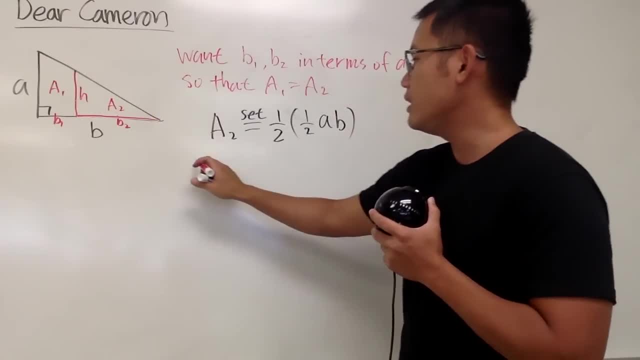 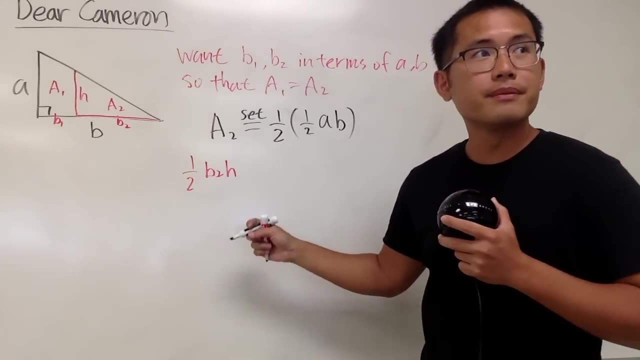 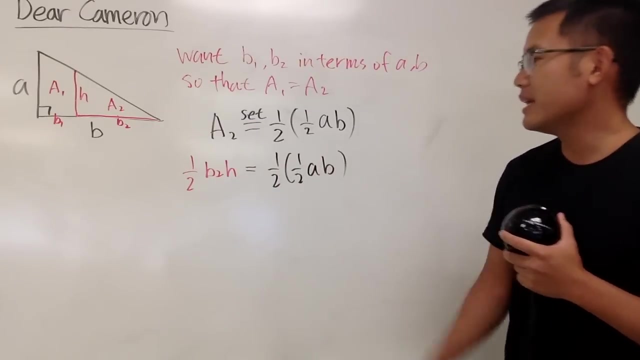 Well, in that case, based on this labeling, A2 will be one half this base times this height, So we just have B2 times H, like this, Anyway. so right, here we were just writing down. this is again one half of one half of AB, right? 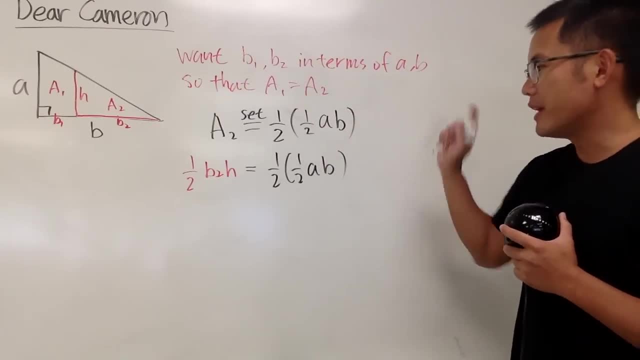 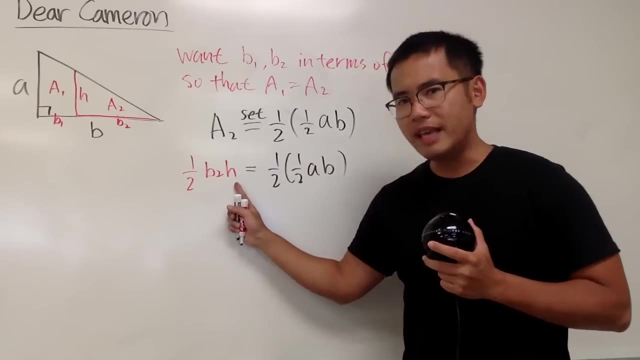 Well, keep in mind, we want to get B1 and B2 in terms of A and B, so our goal is perhaps to try to solve for B2 right here. Hmm, in that case, we don't really want this. H right. 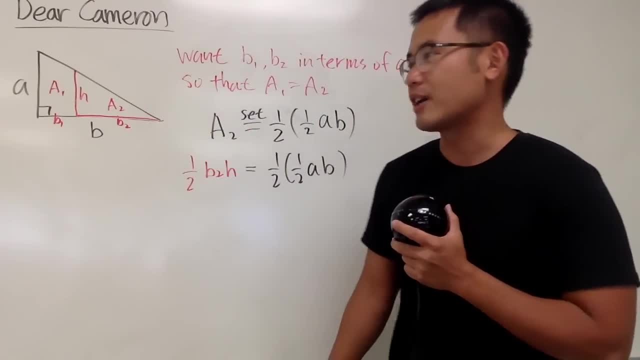 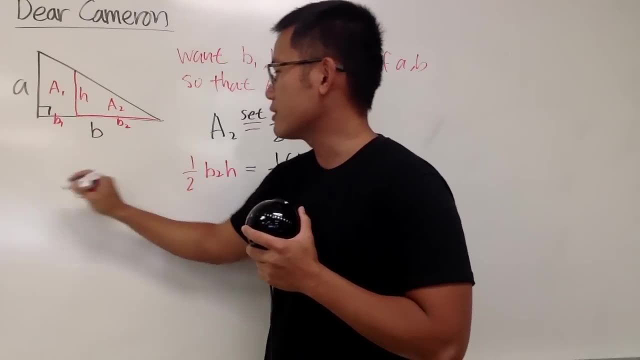 So let's look back to this picture again to see if we can come with any connection so we can get rid of the H, And the connection is similar triangle. So if you guys look at the big triangle in black, so I'll just put this down right here again for you guys. 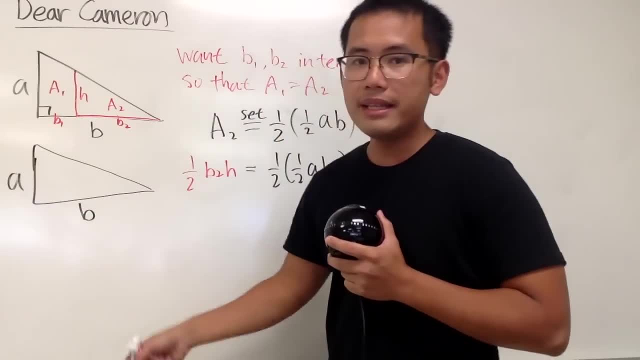 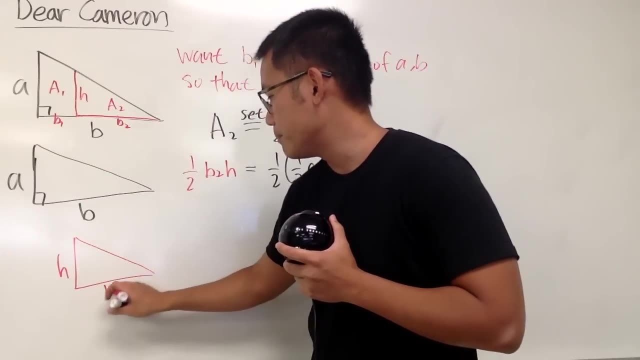 like this: We have A, B right And if we look at the right triangle in red, which is right here, and as you can see, we have H and B2.. Well, in this case, as you can see, 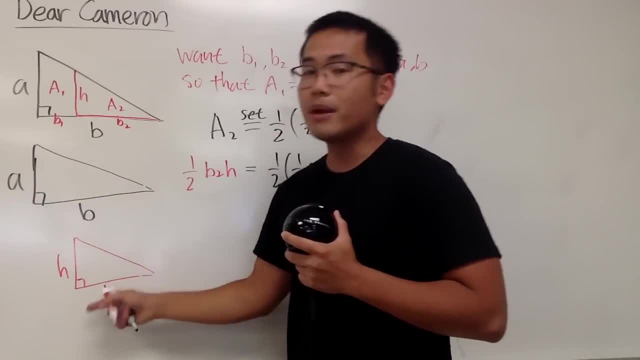 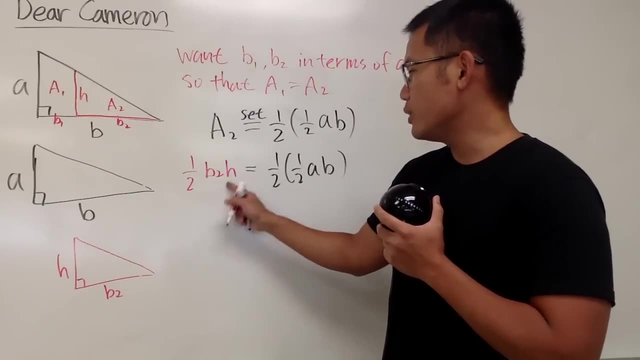 because this angle and that angle are the same and of course they are the same, so by AA they are similar And in that case we can just set up a proportion. and I want to get rid of the H, So let me do H over B2.. 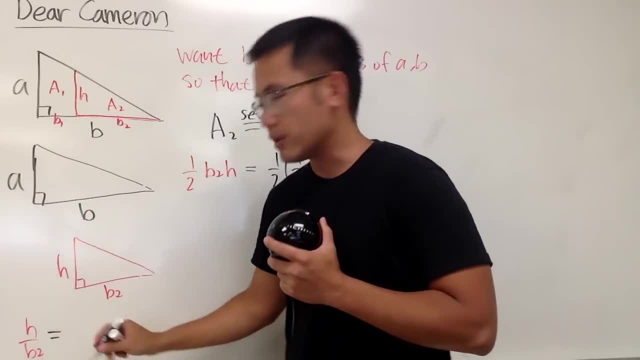 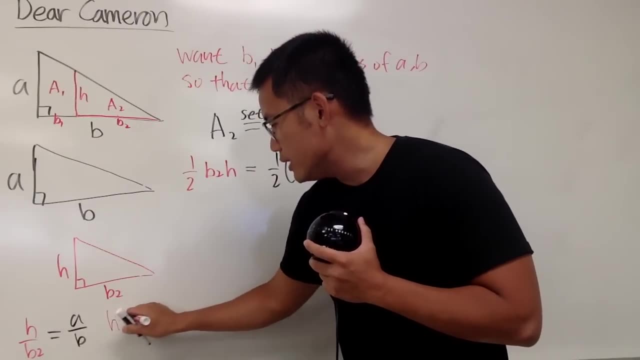 This right here will be the same as A over B. so let's just put that down right here And I will just multiply both sides by B2, so that means H is equal to A over B times B2.. So that way we don't need to see the H anymore. 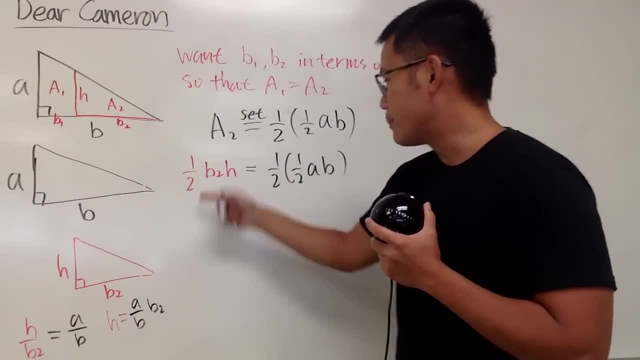 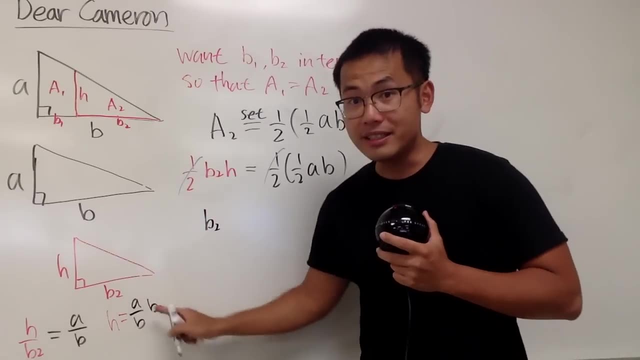 Now we'll come back, Of course. this right here is 1 half, and perhaps we have 1 half 1 half. Let's just get rid of the 1 half on both sides. Here we have B2, and the H is this: 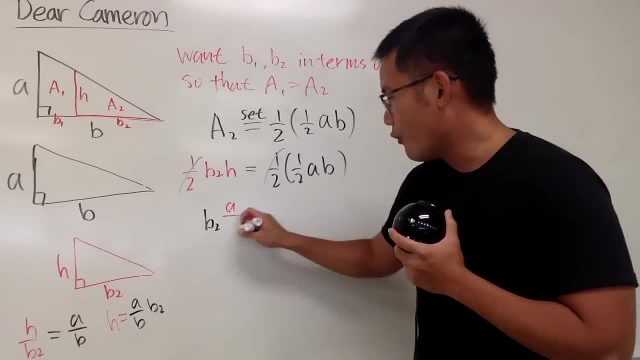 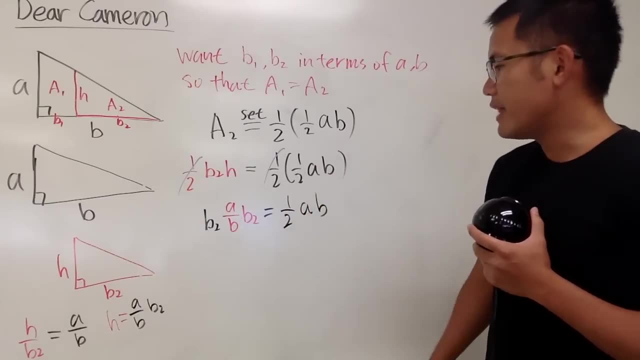 So I will just multiply it by this right here, which is A over B times B2, and the right hand side is 1 half AB, And now let's see if there's anything else that we can cancel. Yes, You see, we have A and A on both sides. 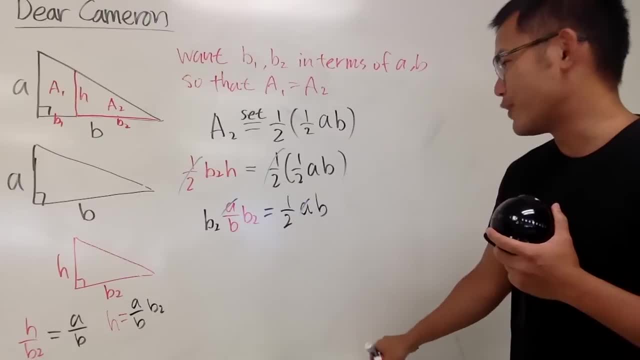 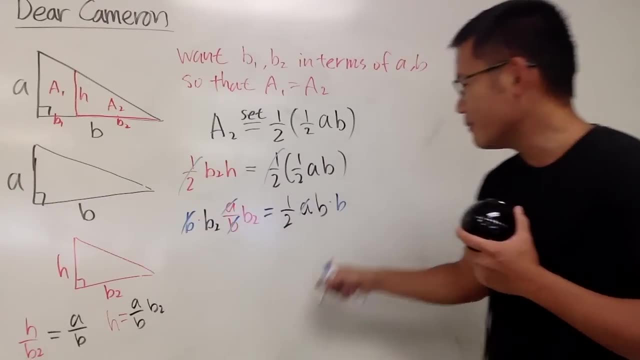 so we can again cancel out like this and that on both sides. That's very nice. And let's multiply B on both sides. So multiply B right here and multiply by B right here, so this and that will cancel, And B2 times B2 is B2 squared. 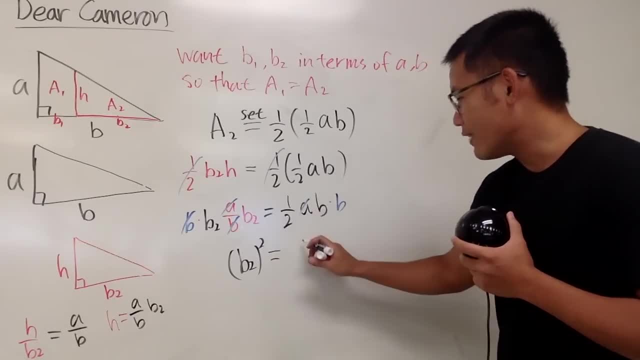 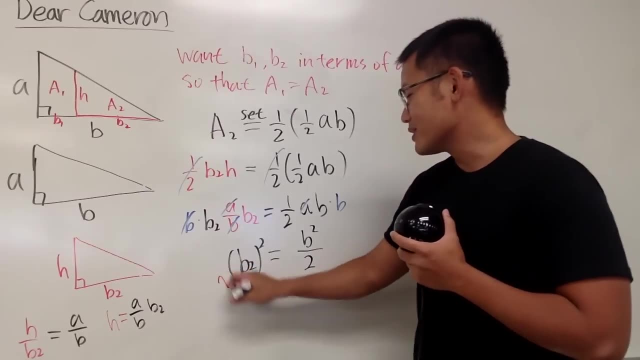 Let me just put it down like this: And on the right hand side we have 1 half, and this is B times B, which is B squared. So just like that, Okay. Now of course, you can just nicely take the square roots on both sides. 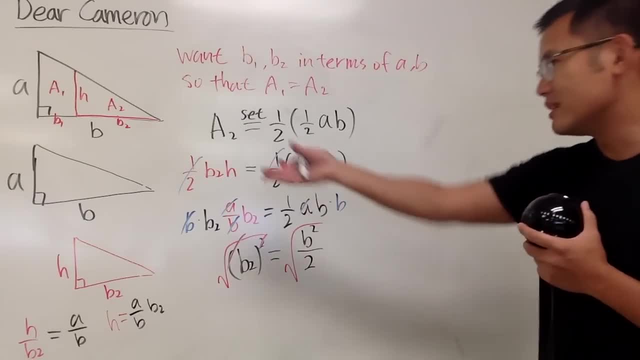 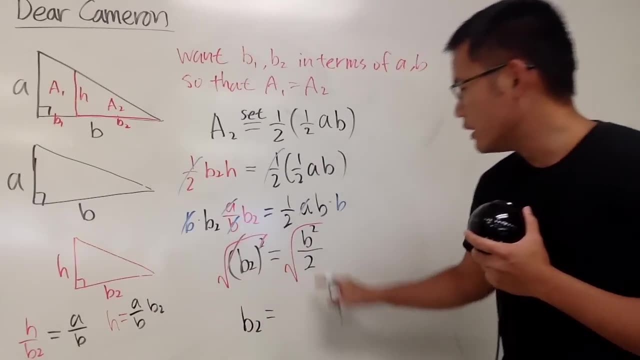 And because we're doing geometry, negative number doesn't make sense in the length right here, so we'll just keep the positive square root only And that will give us B2 equals square root of B. squared is just B over square root of 2.. 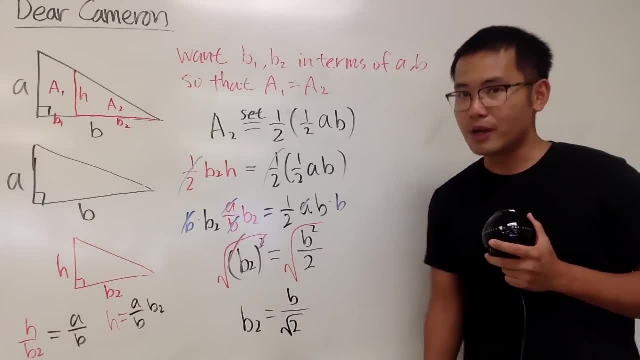 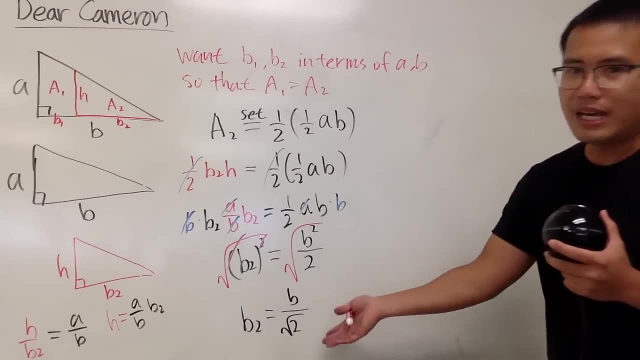 And let's just keep the square root in the denominator, right? So hopefully that's okay. That's pretty much the idea, Because we got a B2. in terms of A and B, Well, there's no A, but the truth is A doesn't matter. 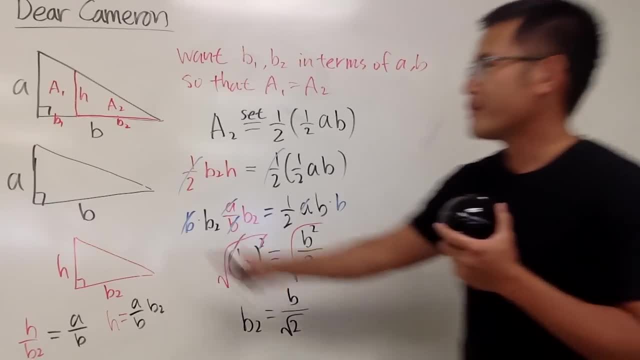 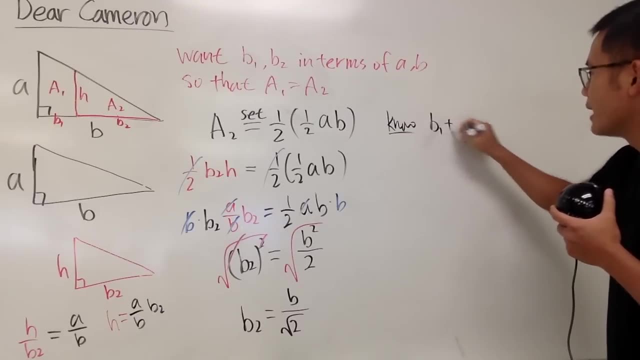 Now we also have to figure out B1 though. So here is the deal: B1 plus B2 is equal to B. We know, Let's put that down. We know B1 plus B2 is equal to B And, of course, B2 is equal to that. 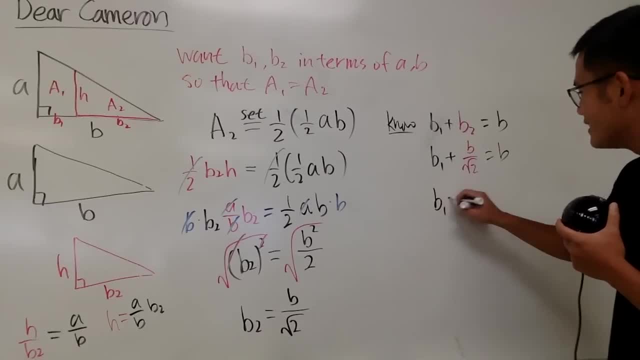 So we know, Of course, minus this on both sides, we see that B1 is equal to B minus B over square root of 2.. So this is actually B2.. So this is actually B2.. So this is actually B2.. 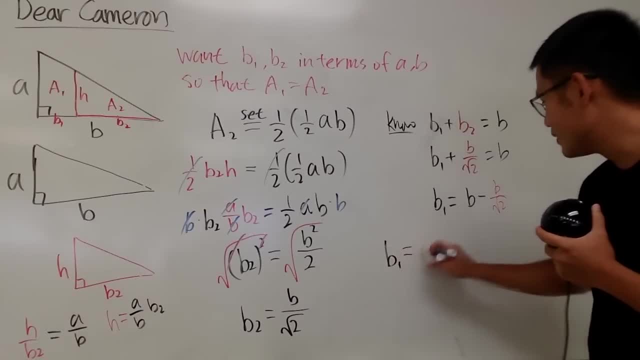 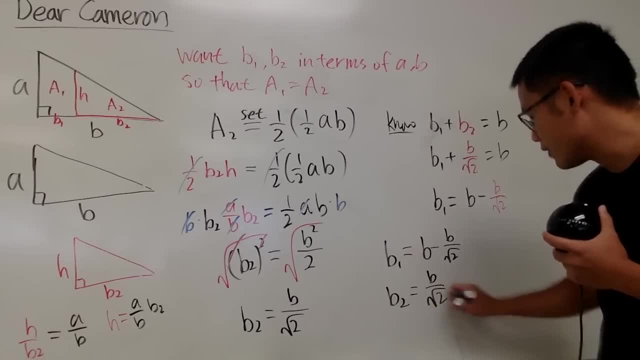 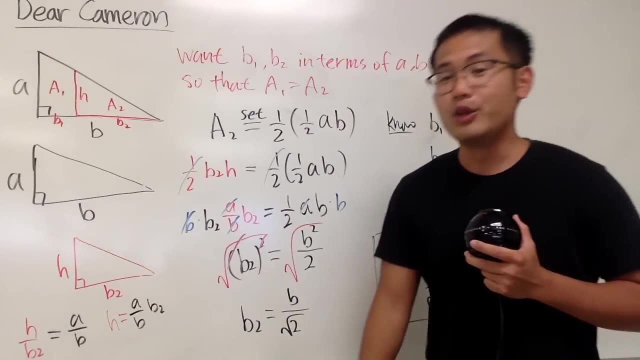 while B2 is just B over square root of 2. So, in fact, A does not matter at all. As long as you measure the B1 and B2 and just make the cut, you will be able to divide the triangle into two pieces. 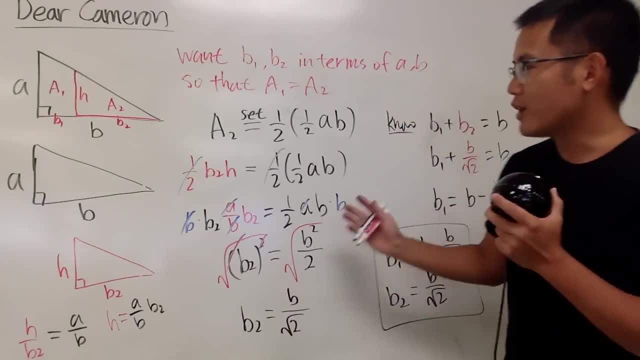 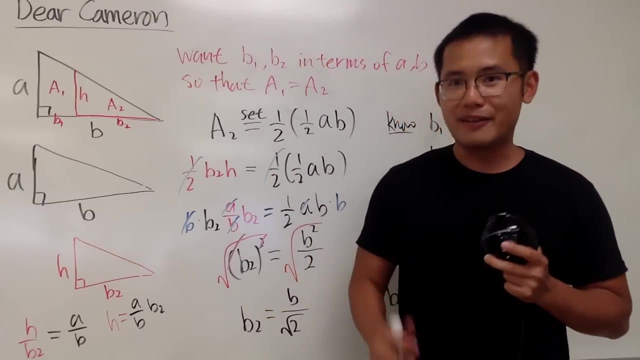 and they will have the same area for both pieces, right, Okay, so hopefully you guys all like this video And Cameron, thank you so much for the question And you're awesome because you're so young and you love math And I like that so much. 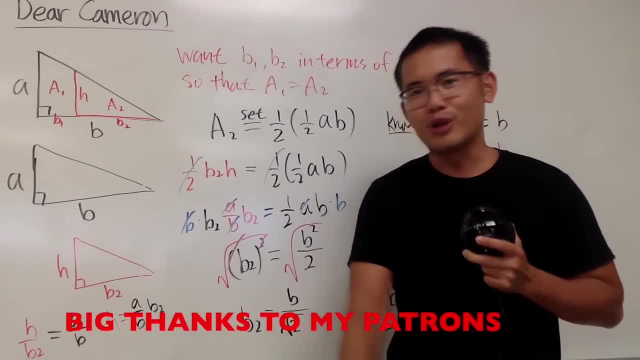 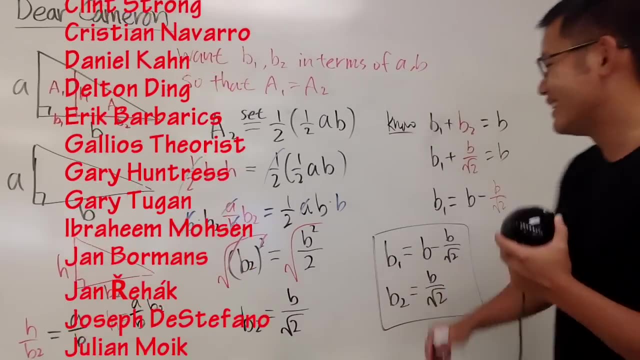 Keep up of your good work and just keep me updated of how you're doing data in the future, right? So I hope to hear more from you later on and just send me more questions if you like. Anyway, that's all And, as always, you know it, that's it.